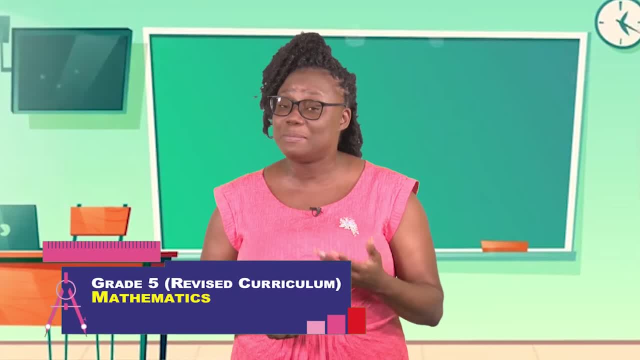 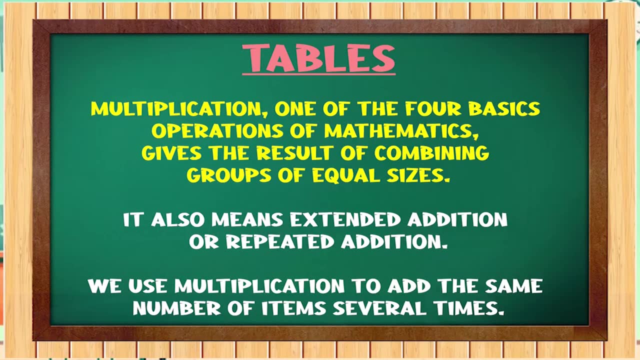 is very essential because it helps you to get your work done accurately and in no time. Multiplication is one of the four basic operations in mathematics. It gives the result of combining groups of equal sizes. It also means extended addition or repeated addition. We use multiplication to add the same number of items several times. 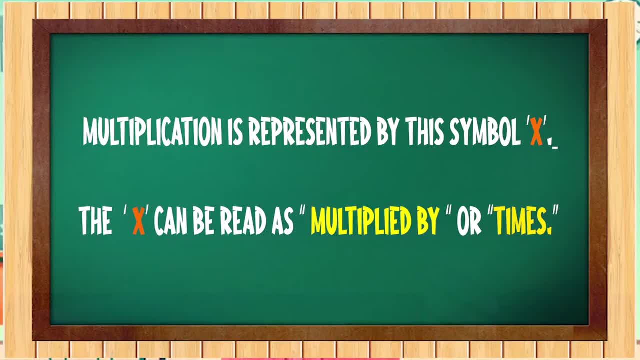 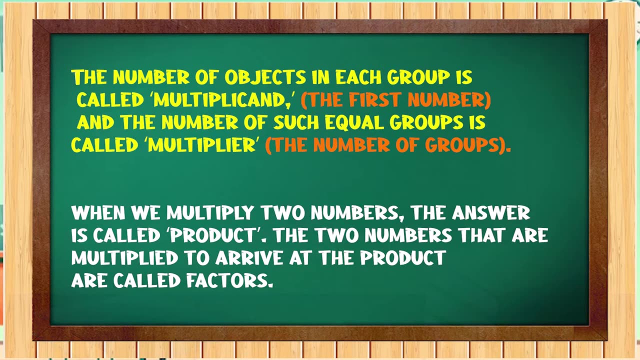 Isn't that cool. Multiplication is represented by this symbol X. It can be read as: multiplied by or times. The number of objects in each group is called the multiplicand. That's the first number in the number sentence And the number of such 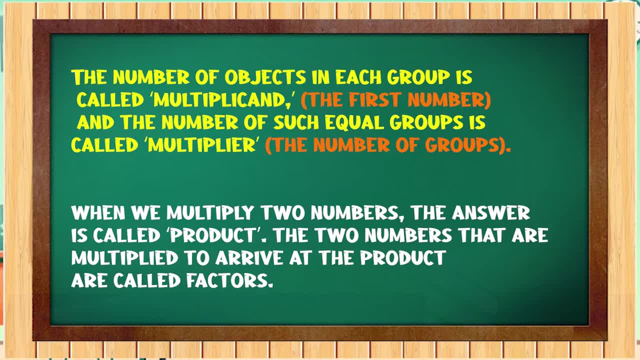 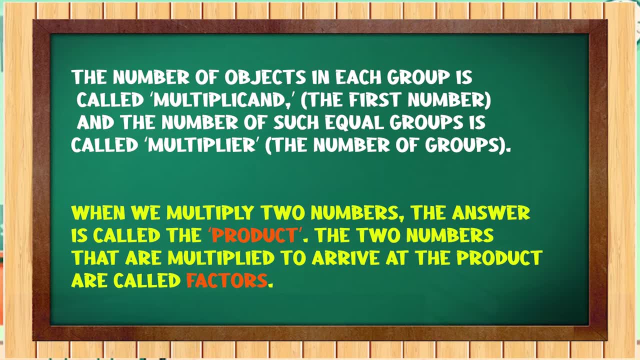 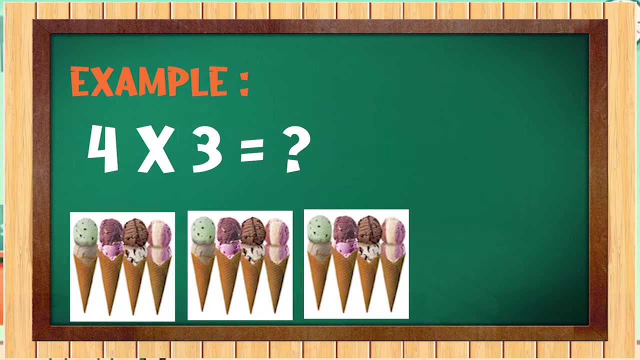 equal groups is called the multiplier. That is the number of groups. That is the second number. When we multiply two numbers, the answer is called the product. The two numbers that are multiplied to arrive at the product are called factors. Let's quickly look at an example. 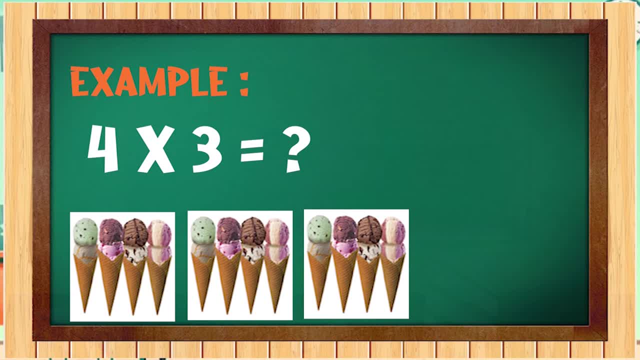 Four times three. The first number is the number of items in each group. You see, there we have some very delicious looking ice cream cones. I love ice cream. Don't you love ice cream? boys and girls, Yes. So we have four ice cream cones in each group. That's the first number. The second number is the 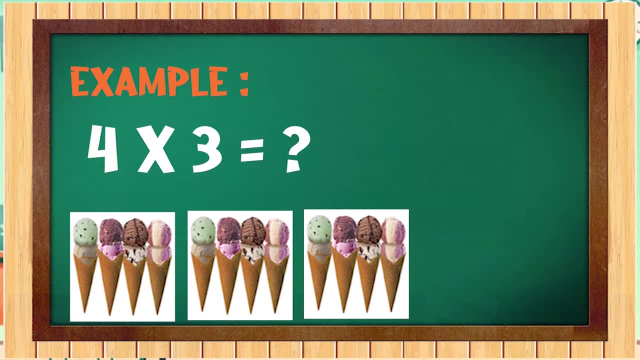 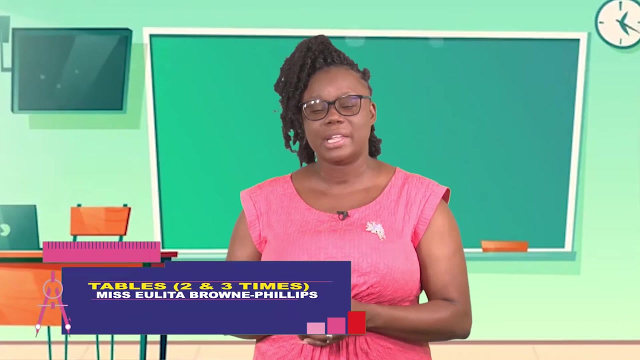 number. then we have three groups. so that diagram represents the number sentence four times three. now we can skip count to find the answer: four, eight, twelve. therefore four times three equals twelve, or four plus four plus four equals twelve. let's quickly look at some multiplication facts. boys and girls, the 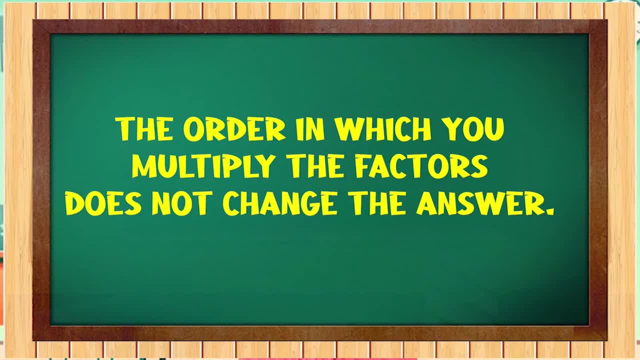 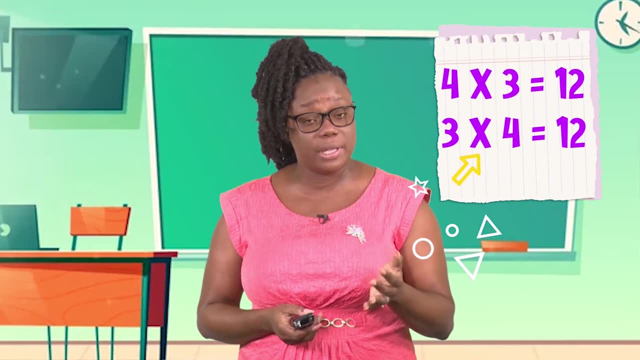 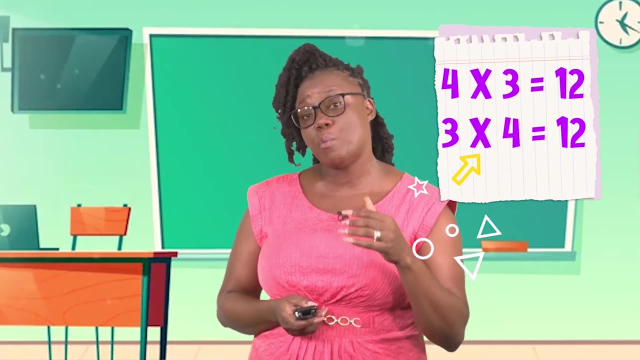 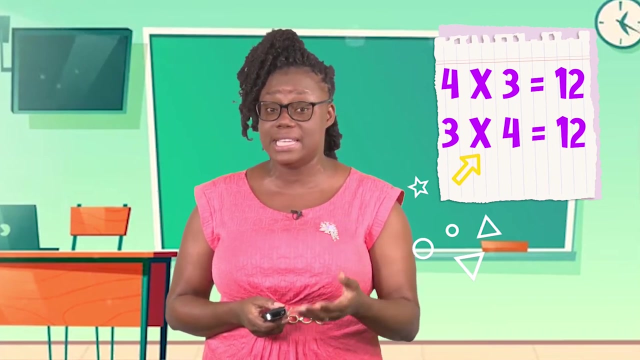 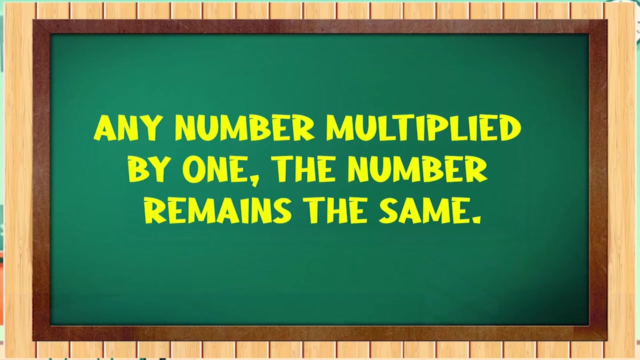 order in which you multiply the factors doesn't change the answer. or four times three will give us twelve, three times four will give us twelve. so it doesn't matter what order the factors are in, the answer or the outcome would be the same. any number multiplied by one, the number remains the same. example four: 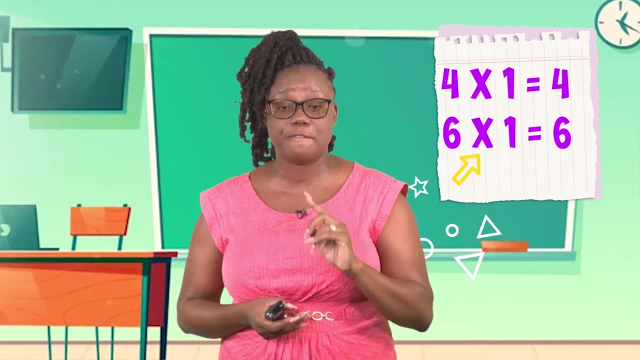 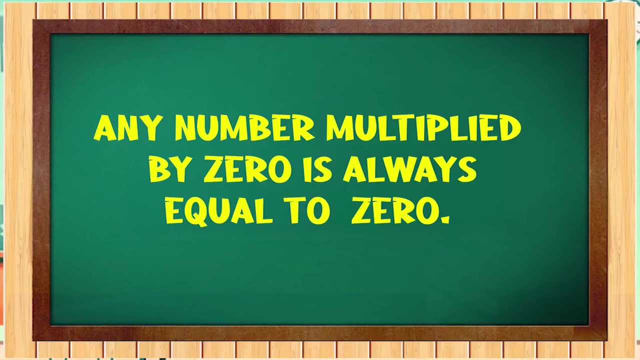 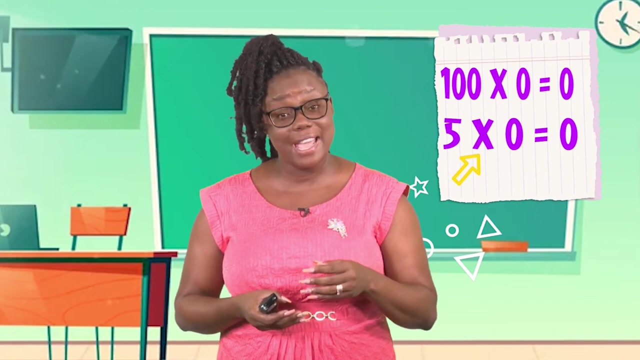 multiplied by one equals four. 6x 1 equals six. any number multiplied by zero is always equal to zero. zero groups of zero will result: and 0 nothing. example: 100 x 0 equals 0. 500 x 0 equals 0. 5X0 equals 0. 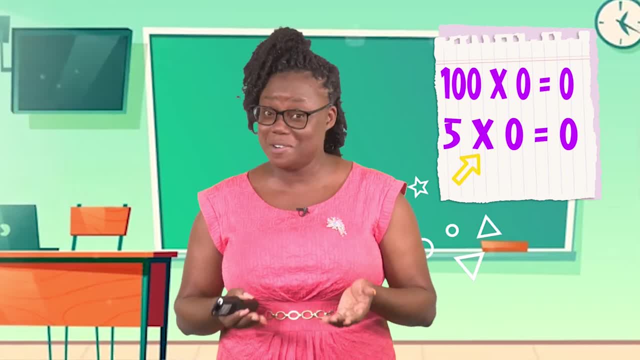 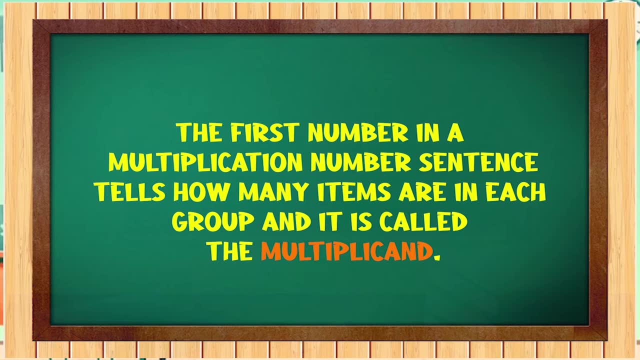 5 x 0 equals 0. X0 equals 0. X0 equals 0 equals zero. of course, the first number in a multiplication number sentence tells how many items are in each group, and it is called the multiplicand. the second number is the multiplier. 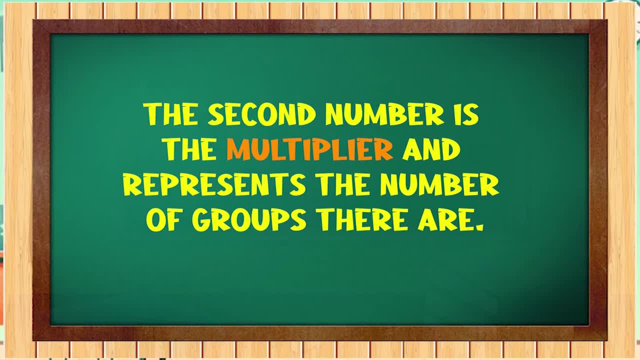 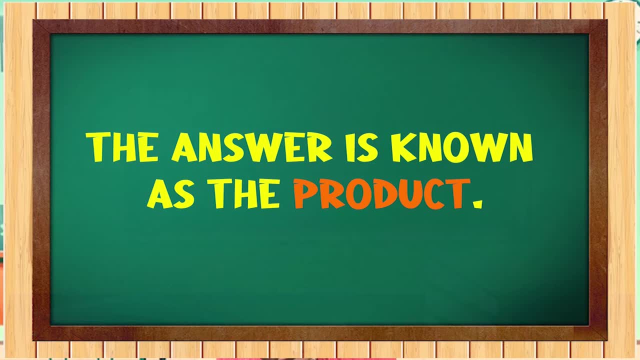 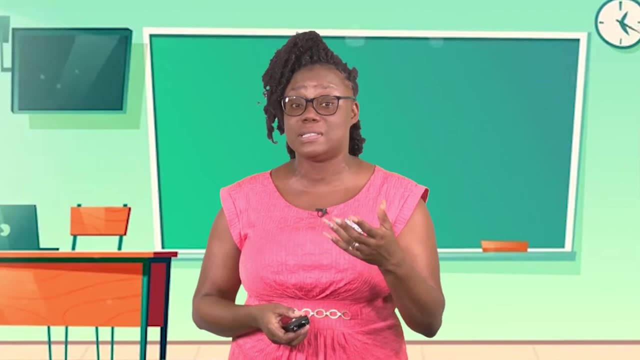 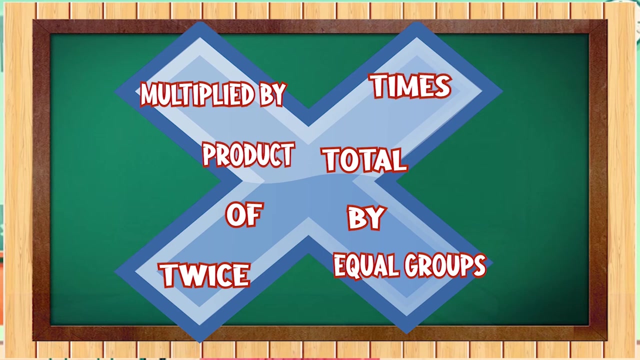 and represents the number of groups there are. the answer, of course, is known as the product boys and girls. let's examine some terms that are associated with multiplication: multiplied by product times, total by equal group groups of, and twice so, once you see these terms appearing in any problem, you should know that you. 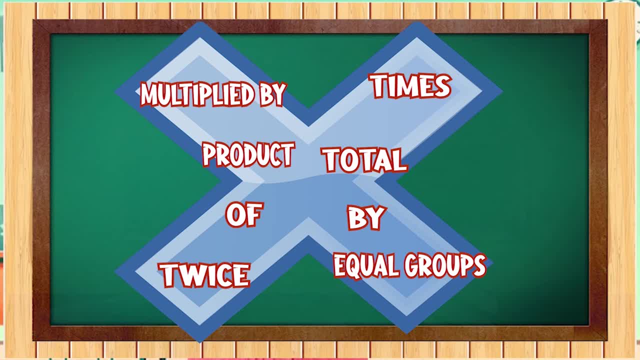 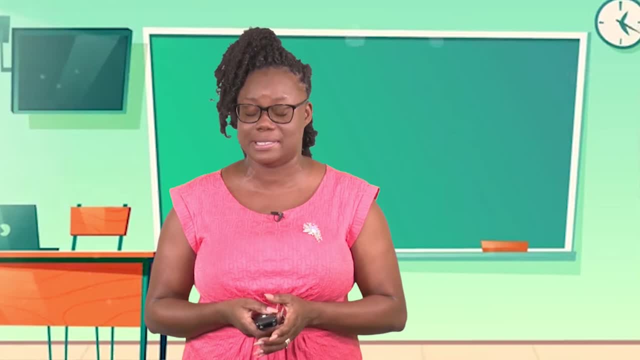 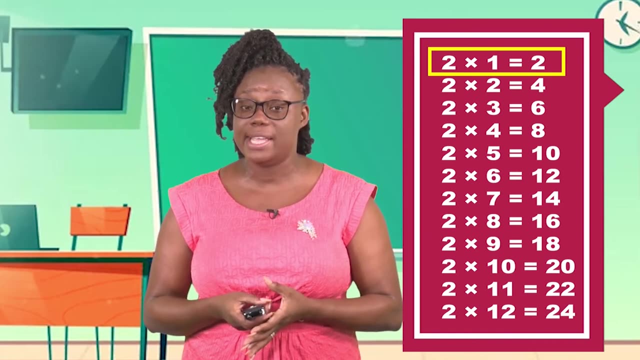 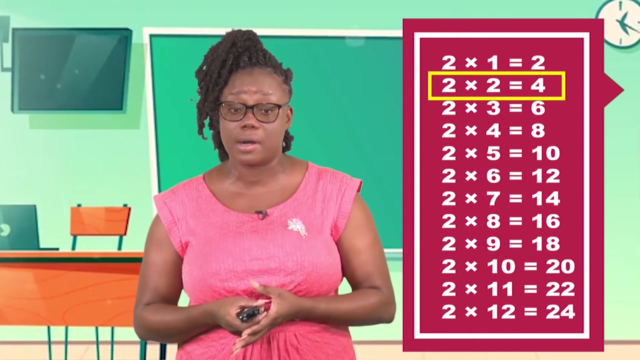 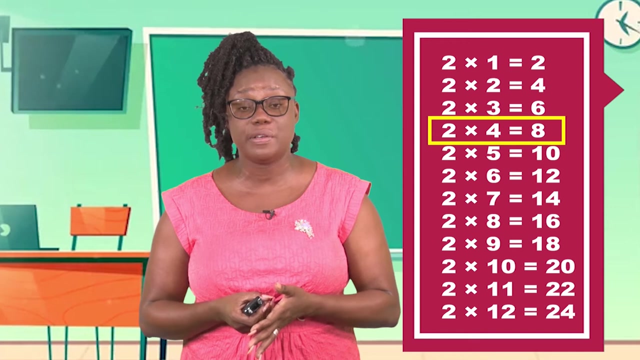 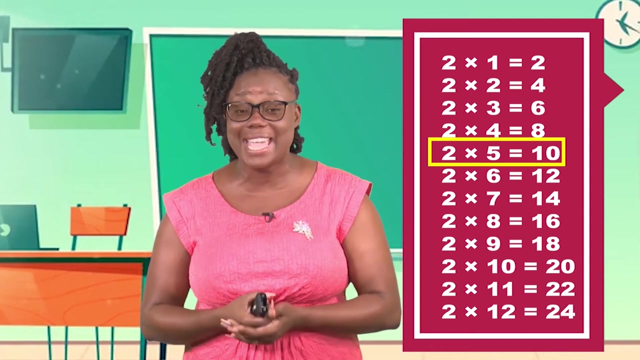 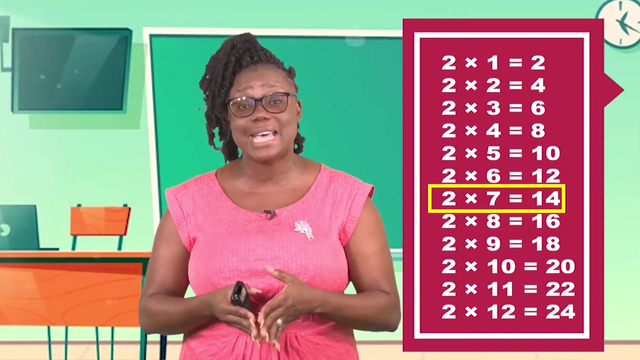 are expected to multiply. now, boys and girls, let's practice our two and three times tables. are you ready? let's go. two times one equals two. two times two equals four. two times three equals six. two times four equals eight. two times five equals ten. two times six equals twelve. two times seven. 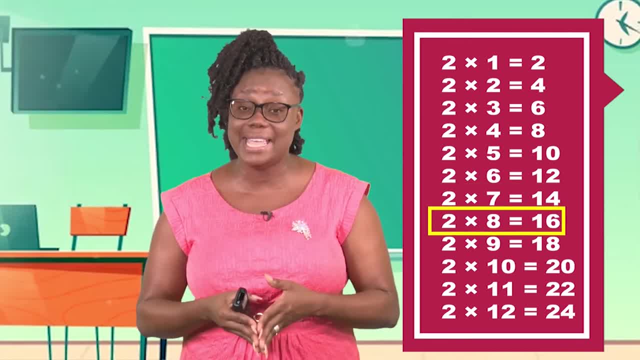 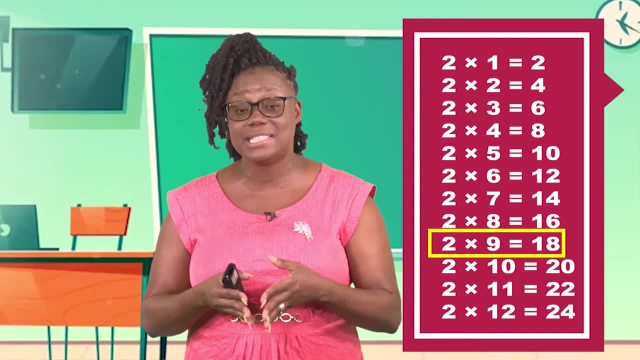 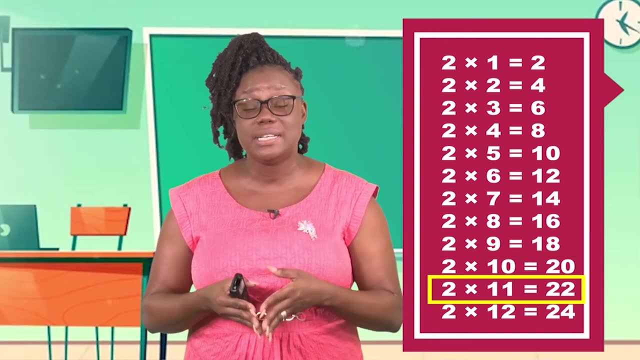 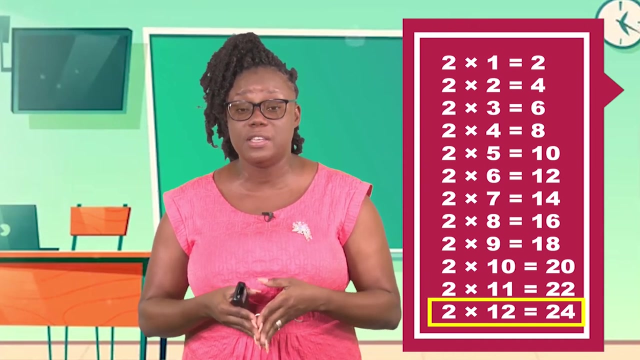 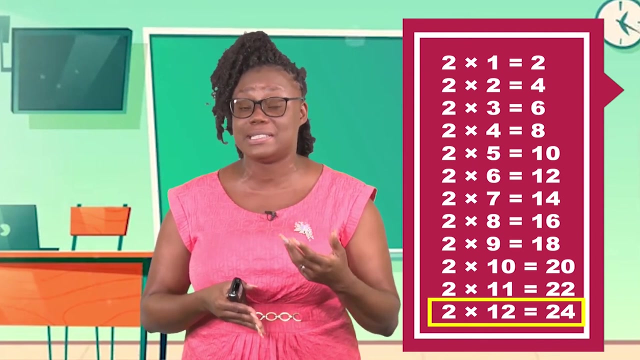 equals fourteen. two times eight equals sixteen. two times nine equals eighteen. two times ten equals twenty. two times eleven equals twenty-two. 2 times 12 equals twenty-four boys and girls. It is very important that we commit our tables to memory. Some people like to memorize it normal, like that. 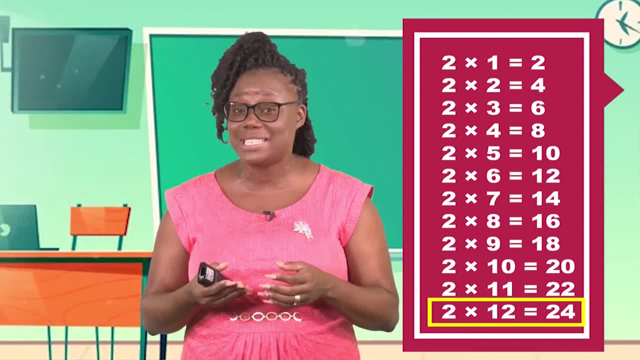 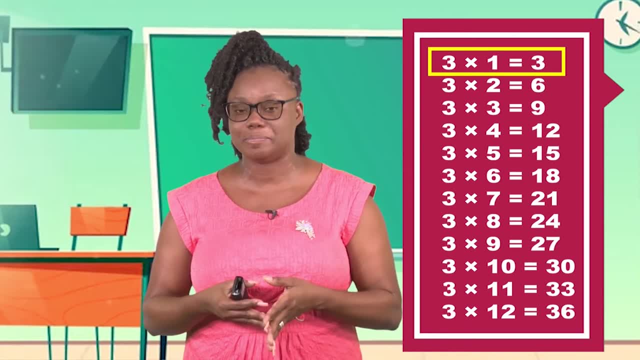 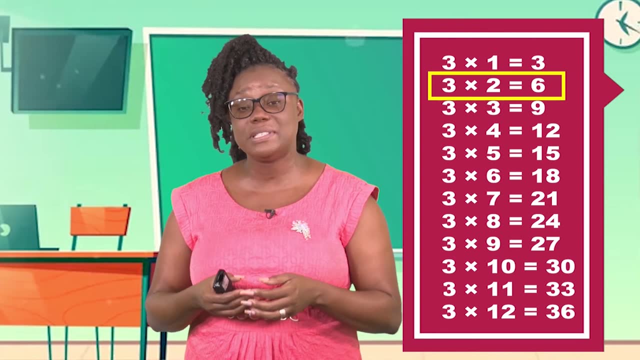 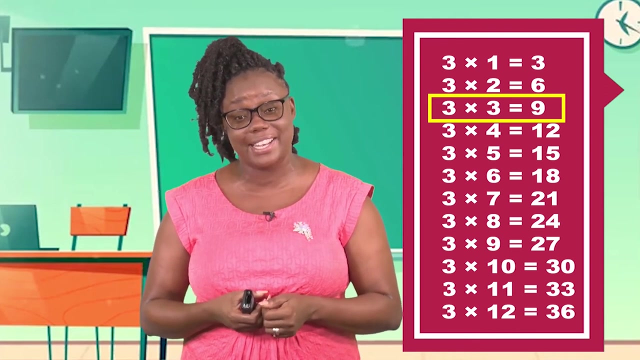 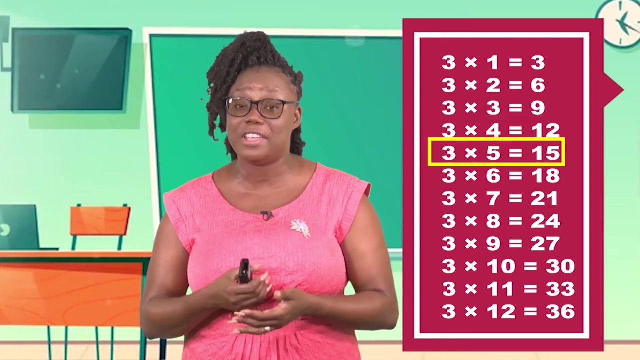 but you can add some type of music to it so that you can remember it. Let's go through our three times tables. Three times one equals three. Three times two equals six. Three times three equals nine. Three times four equals twelve. Three times five equals fifteen. 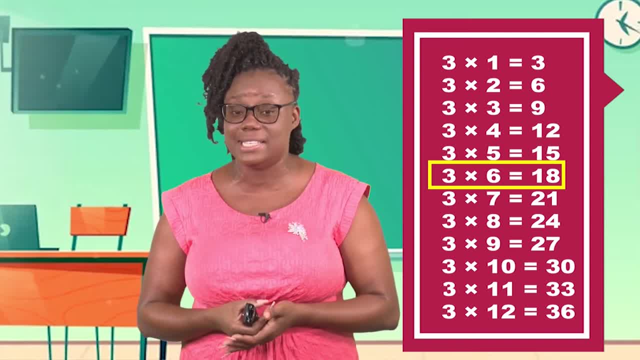 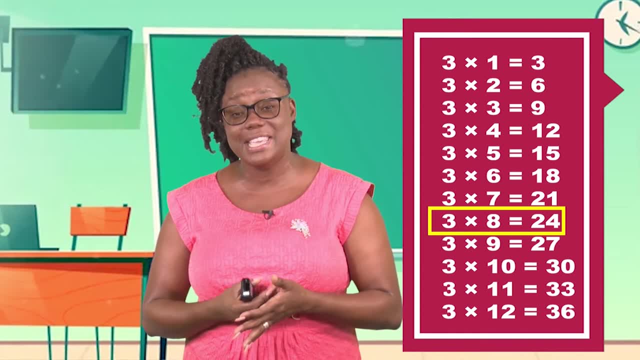 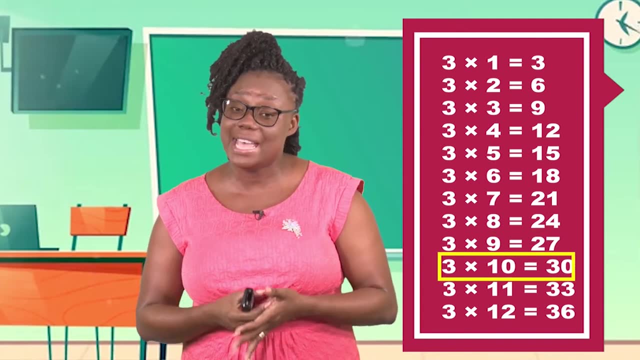 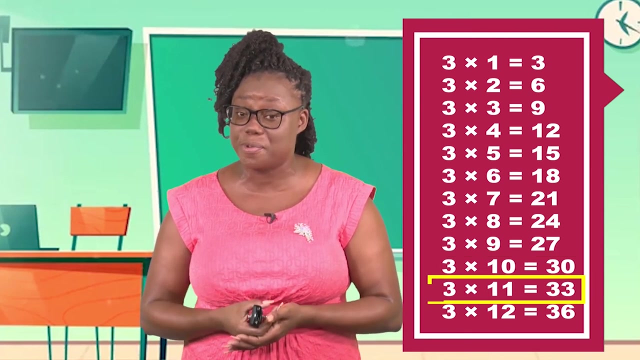 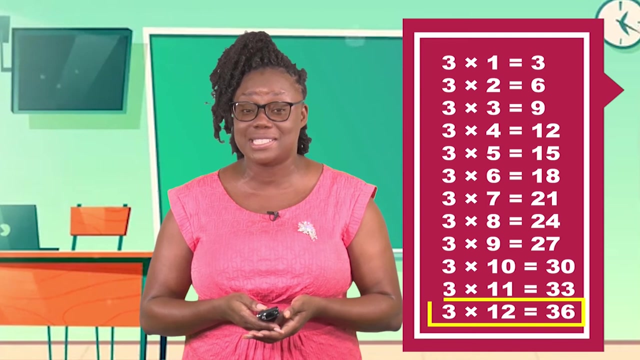 Three times six equals eighteen. Three times seven equals twenty-one. Three times eight equals twenty-four. Three times nine equals twenty-seven. Three times ten equals thirty. Three times eleven equals thirty-three. Three times twelve equals thirty-six. Excellent job, boys and girls. 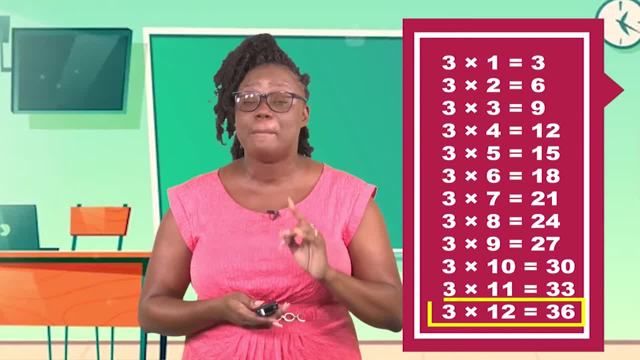 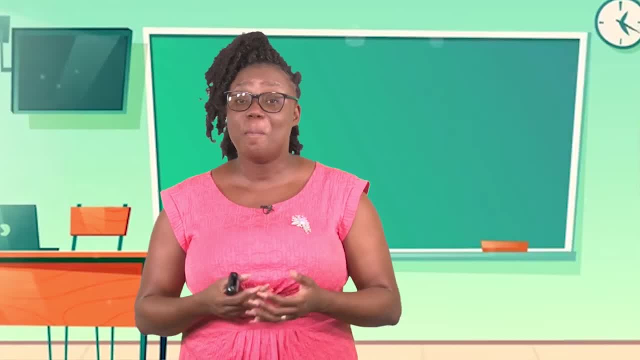 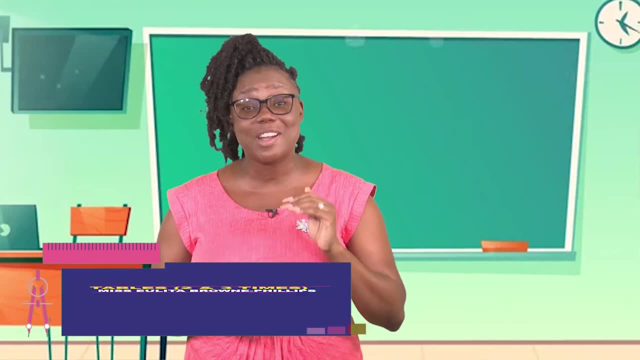 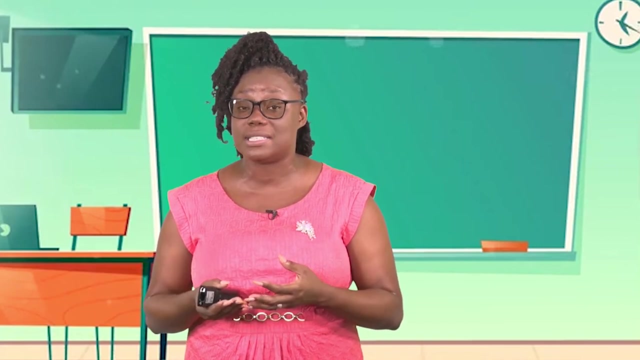 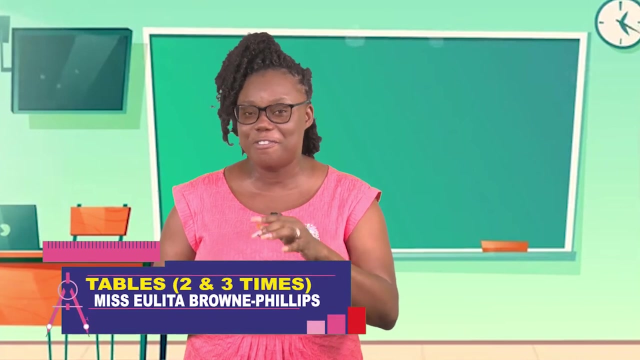 Remember to commit your tables to your memory, because it will help you when you are solving mathematical problems. Boys and girls, this has brought us to the end end of today's lesson. I trust that you will be good multipliers from today onwards. we are about to bring the curtains down, but we never bring the. 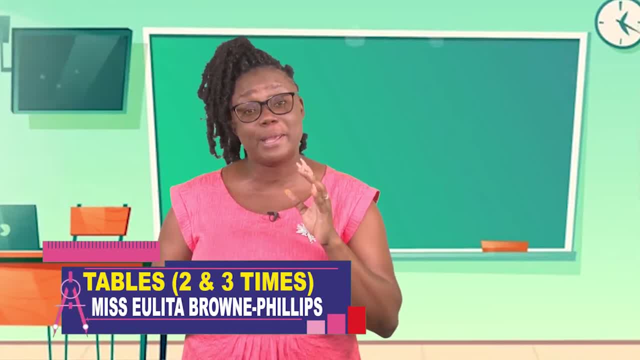 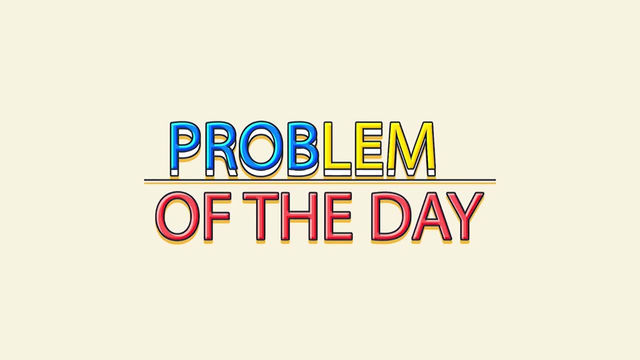 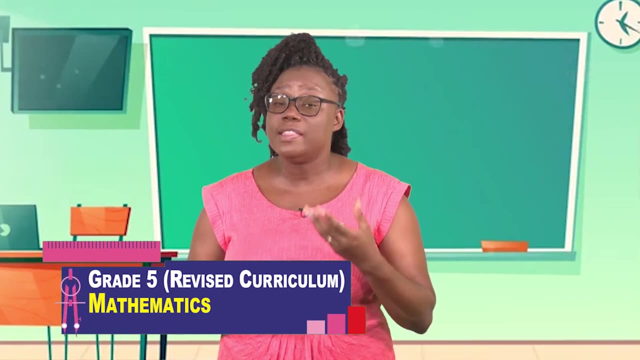 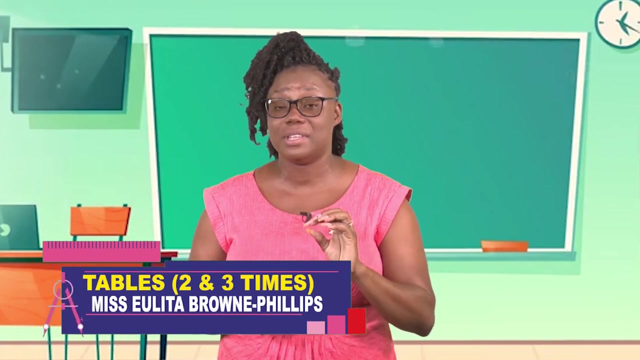 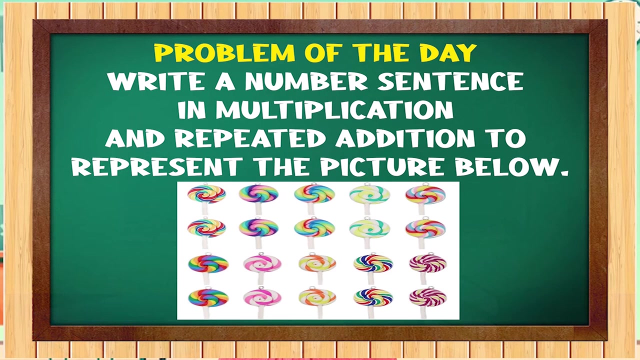 curtains down without giving our little problem solvers the problem of the day to solve. Jim was very, very sad. he could not multiply. I want you to help Jim look at the pictorial representation and write a number sentence in multiplication and repeat it again: addition to represent the picture. are you gonna help Jim? yes, boys and girls, I 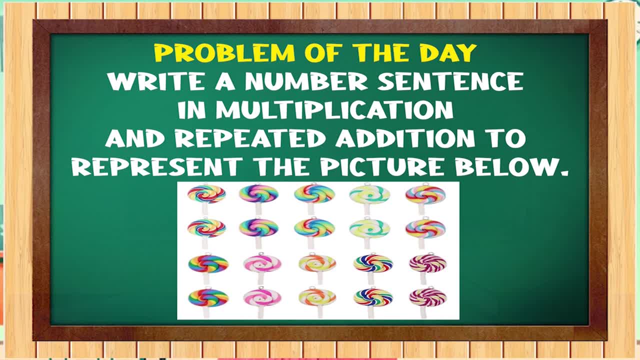 know you are excellent problem solvers. take a few seconds and get this done. I hope you enjoyed this video. if you did, please give it a thumbs up. if you liked this video, please subscribe to my channel and hit the bell icon, so you don't miss out on any of my future videos. 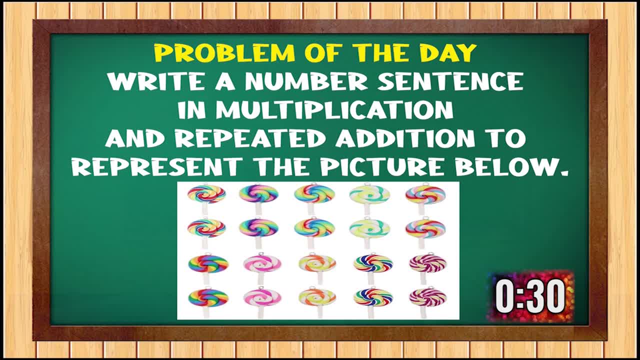 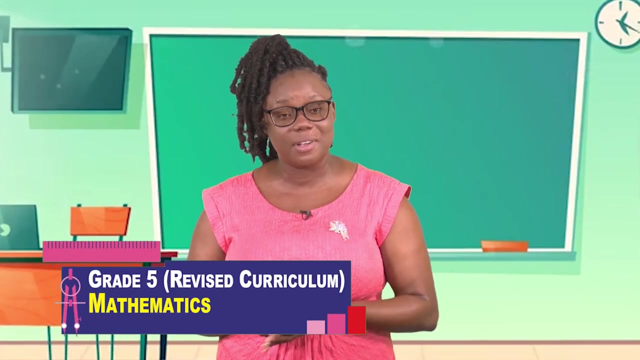 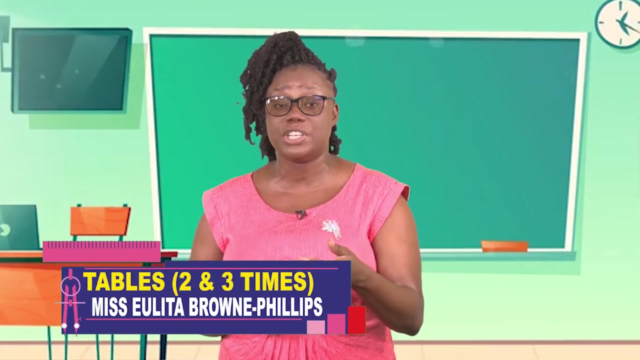 thank you so much for watching and I'll see you in the next video. bye, bye. you should be finished by now. let's look at the problem. you had to write a number sentence in multiplication and one in repeated addition. let's tackle the one with multiplication on it. 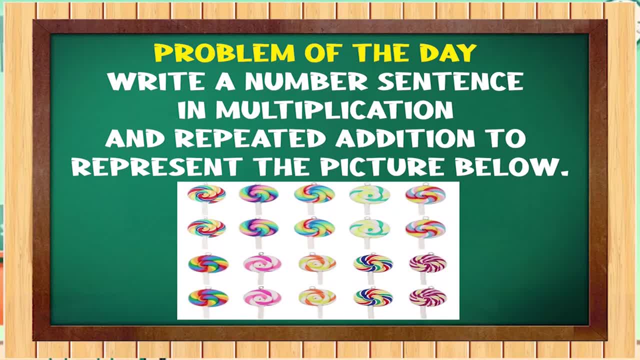 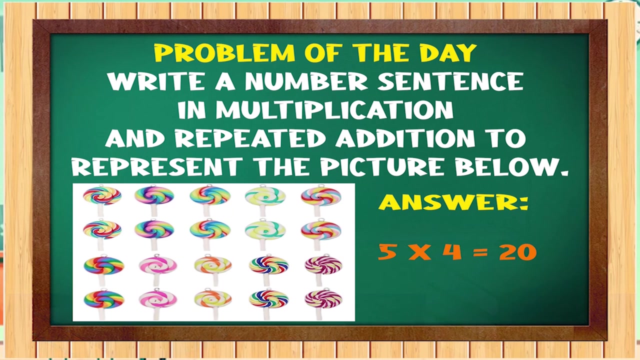 let me soon inki section. that were. what a slipped multiplication. first, what are you seeing there? we have some lollipops. we have four rows of five lollipops. which number will go first? five? the first number is five and that five represents the amount of lollipops in each group. how many groups are there? four? so five times four equals. 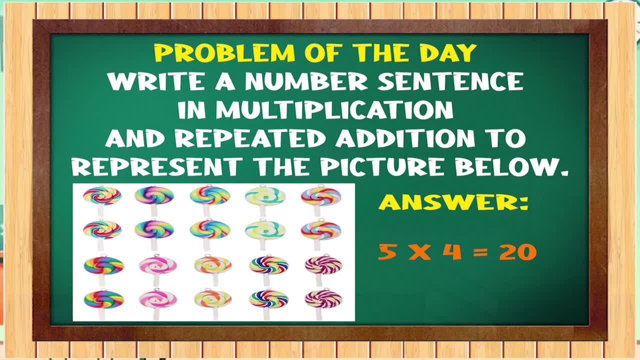 twenty boys and girls. it can be written another way. let's flip this and write it another way. we can also have four, four lollipops in each group. how many groups do we have of four lollipops? five groups of four lollipops. so that is the number sentence. 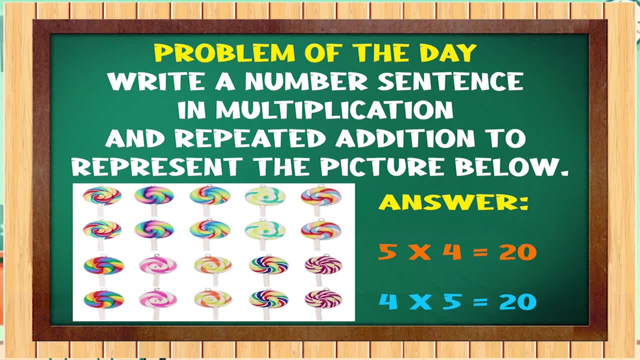 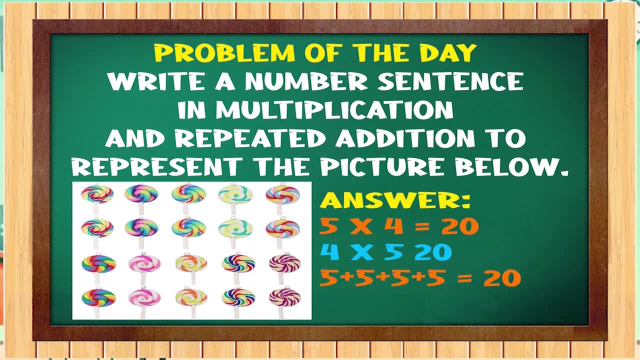 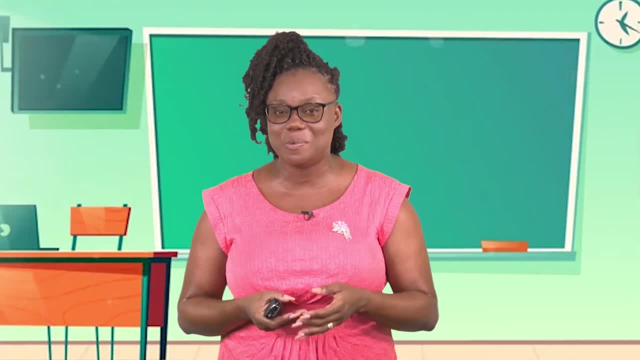 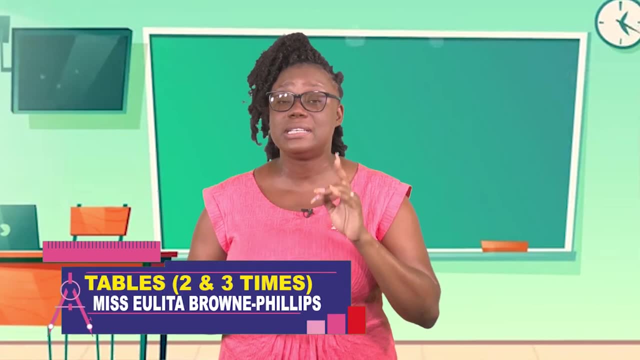 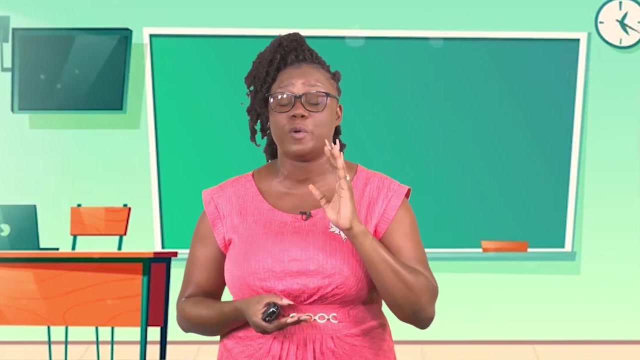 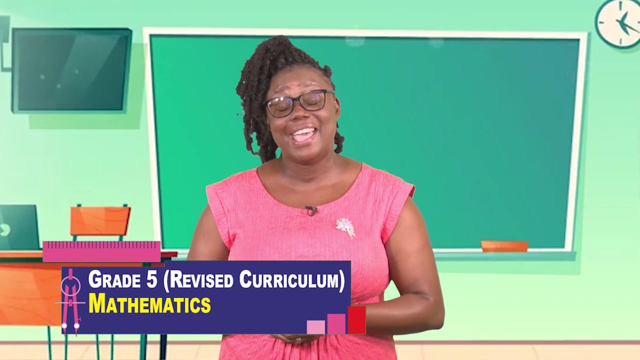 have that answer. Excellent work. I am beyond proud of my little multipliers. So, boys and girls, remember to commit your tables to memory so that it will help you to solve your problems in the quickest time possible. I want you to remember, boys and girls. it was Dan Waldschmidt who said: 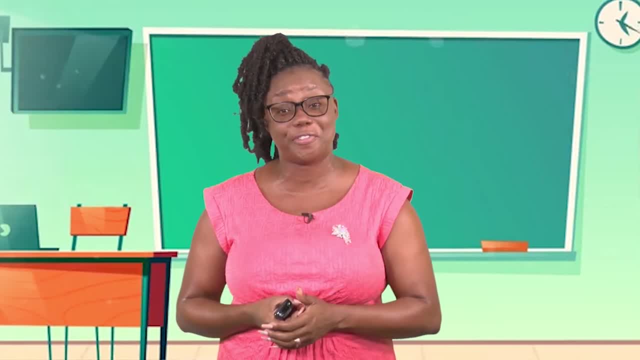 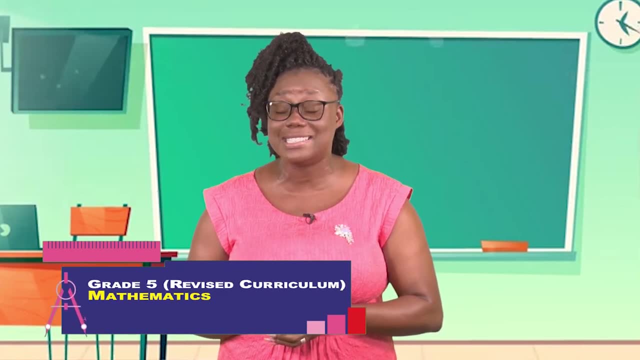 if you have to give up. give up on your fear, Give up on your fear of mathematics. Thank you for joining us today. boys and girls, See you next time.